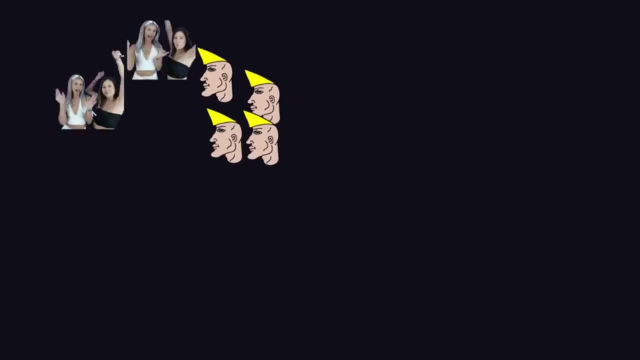 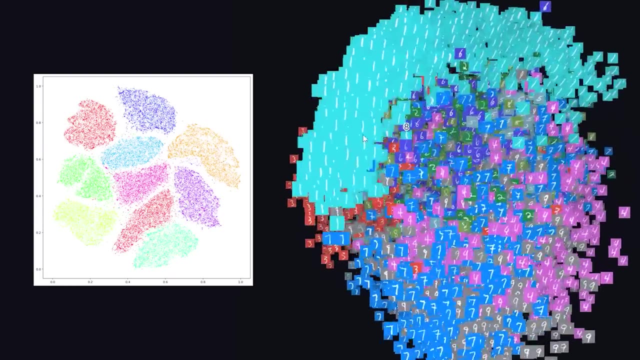 Meanwhile, all the girls find the dance floor. while you group together with all the programming introverts to talk about vectors in the corner, Notice how all the similar objects are grouped together. Embeddings work the same way, except they map the semantic meaning of words together. 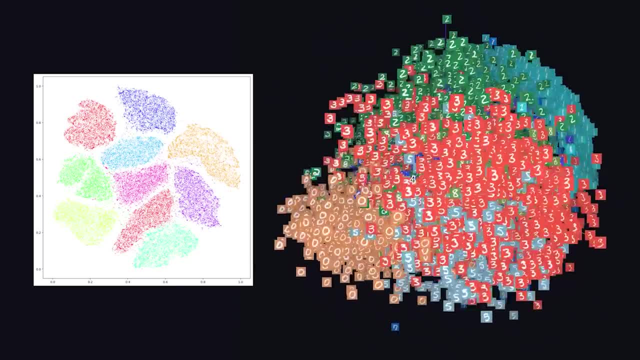 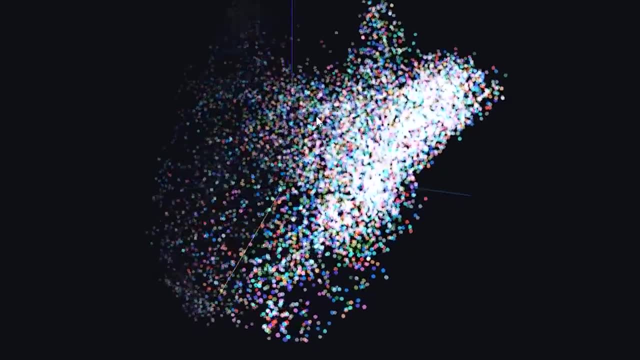 or similar features in virtually any other data type. These embeddings can then be used for things like recommendation systems, search engines and even text generation, like ChatGPT. But once you have your embeddings, the question becomes: where do you store them and how do you query them quickly? 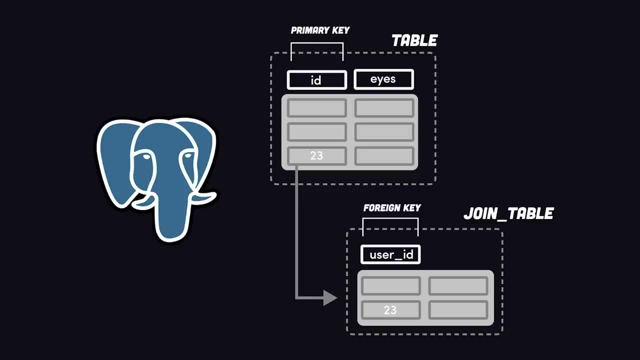 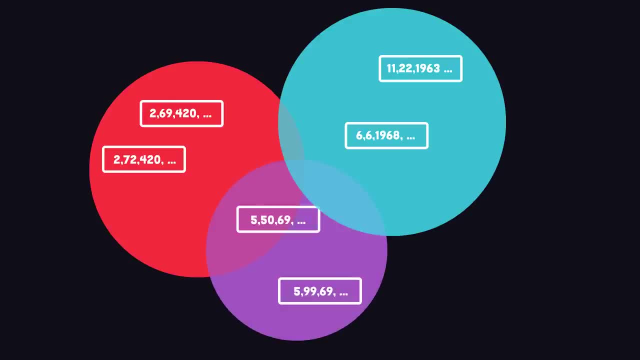 That's where vector databases come in. In a relational database, you have rows and columns. In a document database, you have documents and collections. But in a vector database, you have arrays of numbers clustered together based on similarity, which can be queried with ultra-low latency. 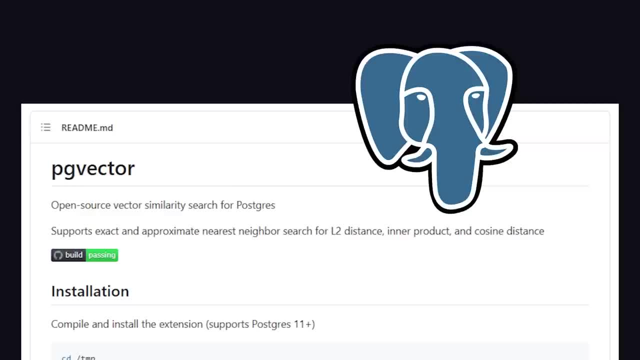 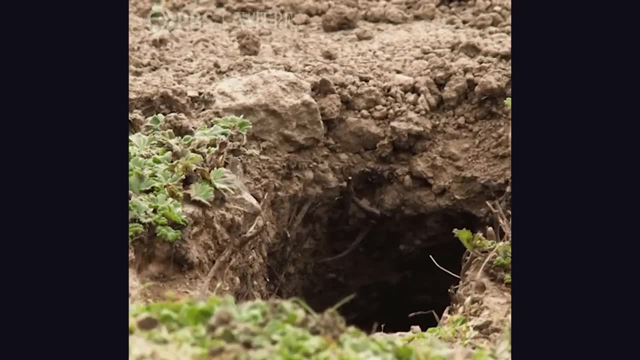 making it an ideal choice for AI-driven applications. Relational databases like Postgres have tools like PGVector to support this type of functionality, and Redis also has first-class vector support. But a bunch of new native vector databases are popping up, like Weeviate and Milvus are open-source options written in Go. 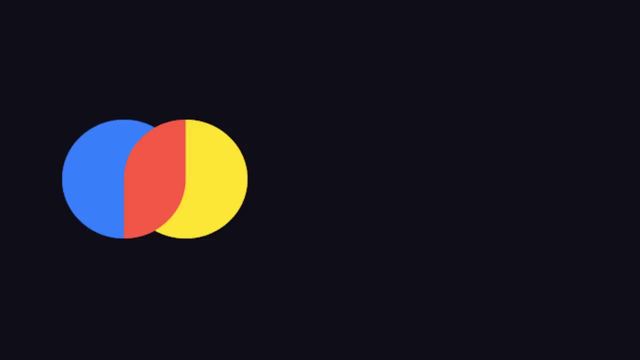 Then you have Pinecone, which is extremely popular but is not open-source. Then you have Chroma, which is based on ClickHouse under the hood, and many other options from there. Let's jump into some code to see what it looks like. 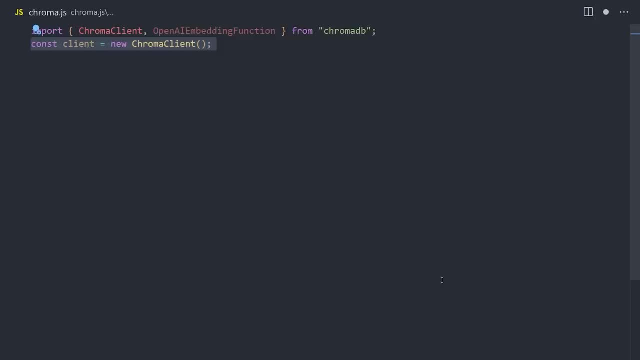 Here I'm using Chroma and JavaScript, and the first thing I'll do is create the client, then define an embedding function. In this case, it will use the OpenAI API to update the embeddings whenever a new data point is added. Each data point is just a document with an ID and some text. 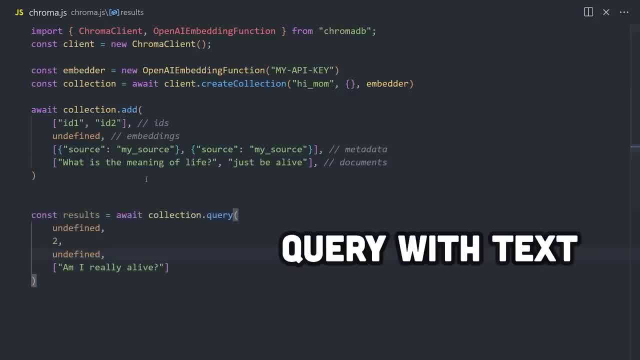 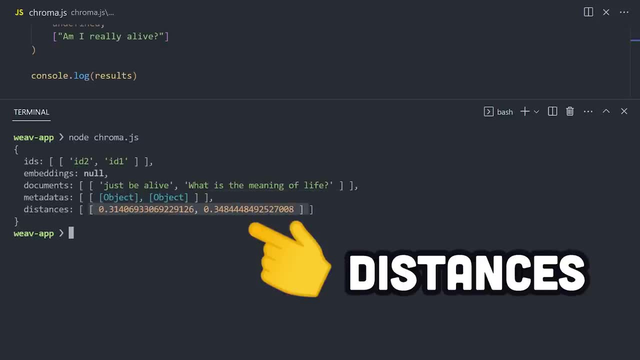 And finally, we can query the database by passing a string of text, just like an LLM. What's most interesting, though, is that in the query result, we get the data back in addition to an array of distances, with a smaller number indicating a higher degree of similarity. 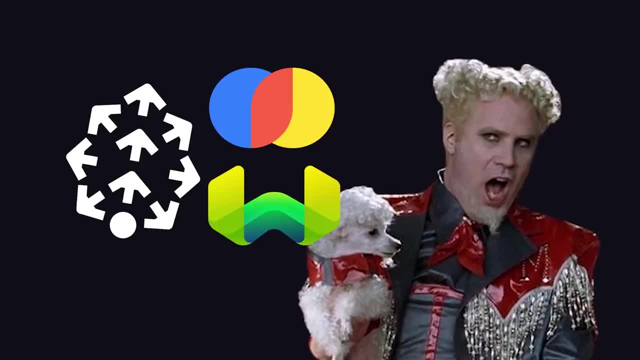 That's pretty cool, but the real reason that these databases are so old is because they're so old. but the real reason that these databases are so old is because they're so old. but the real reason that these databases are so old is because they're so old. 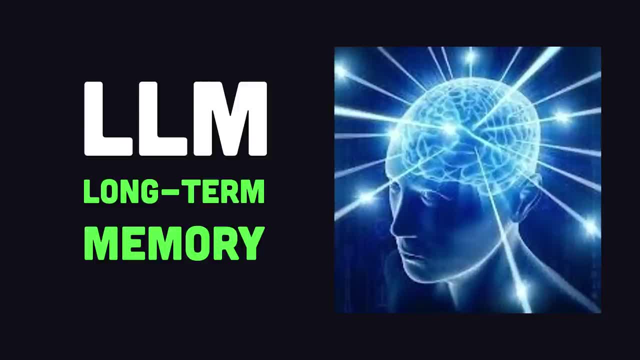 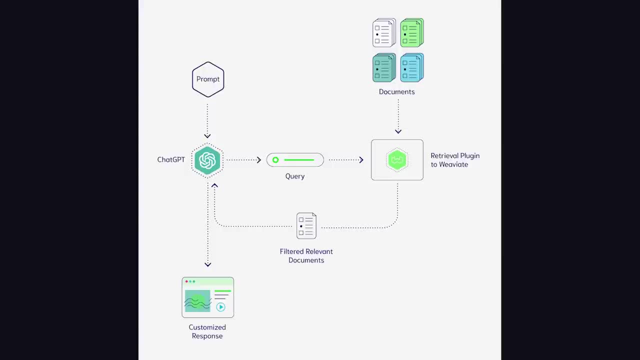 is that they can extend LLMs with long-term memory. You start with a general-purpose model like OpenAI's GPT-4, Meta's Llama or Google's Lambda, then provide your own data in a vector database. When the user makes a prompt, you can then query relevant documents from your own database to update the context. 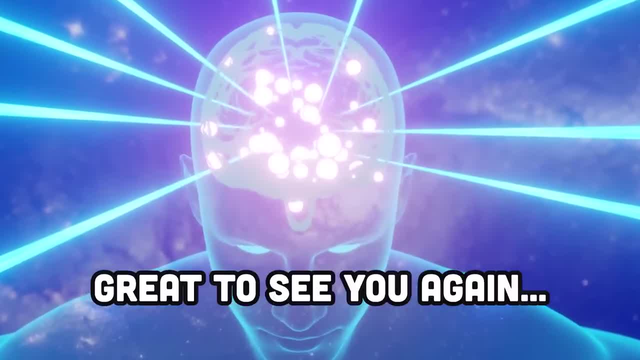 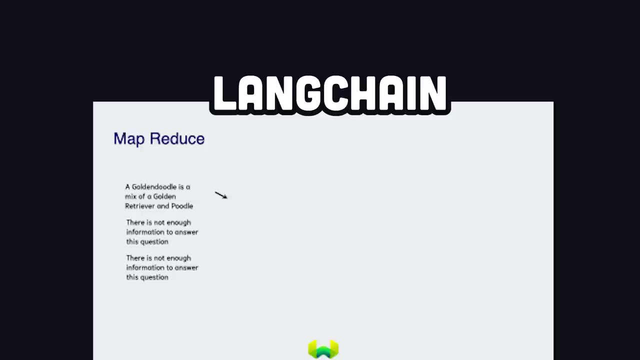 which will customize the final response, And it can also retrieve historical data to give the AI long-term memory. In addition, they also integrate with tools like Langchain that combine multiple LLMs together. It's all pretty crazy, and I'm working on a tutorial on my second channel with Weevy8,.